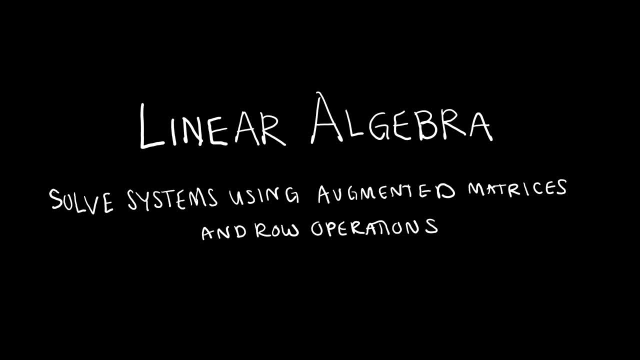 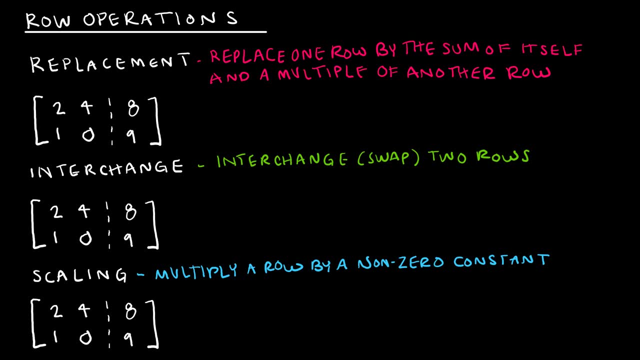 and talk about what our possible row operations are: what's legal, what's illegal, etc. We have three row operations to choose from. The first is called replacement, and replacement tells us that we can replace one row by the sum of itself and a multiple of another row. 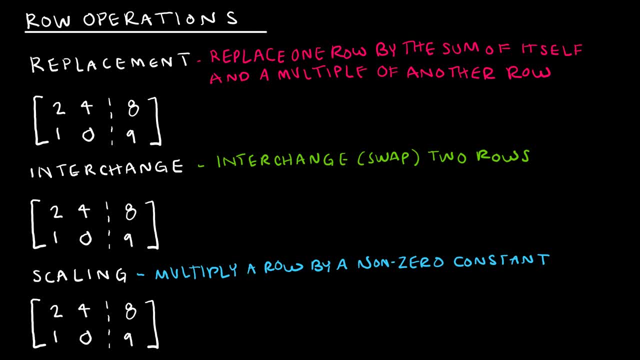 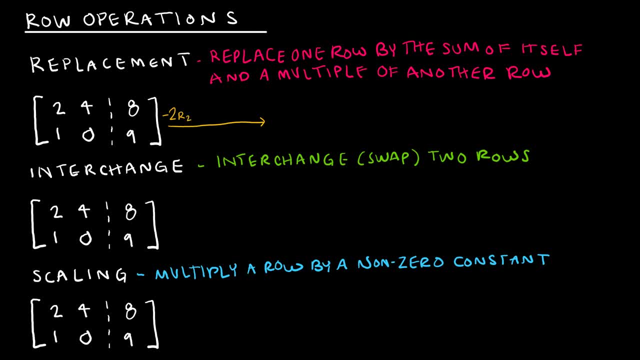 So we're going to take row two, which of course is going to turn this into negative two and zero and negative 18, and perhaps I'll want to add that to row one, And then- this part's very important- I'm going to say the target row. So where is this going to land When I add negative two times row? 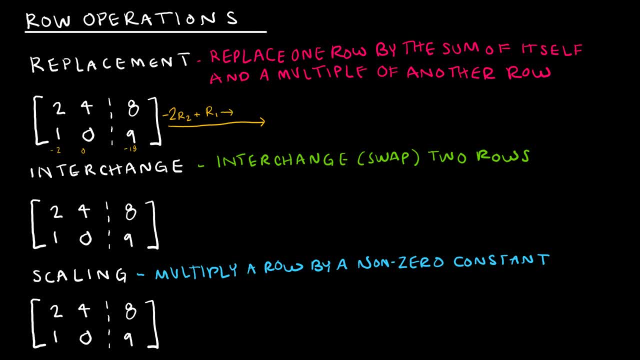 two to row one. is that going to replace row one or is it going to replace row two? And in this case, let's say it's going to replace row 2. what that tells me is row 1 is still going to be 2, 4, 8, but row 2 is now. if I take negative 2 times row 2 and add it, 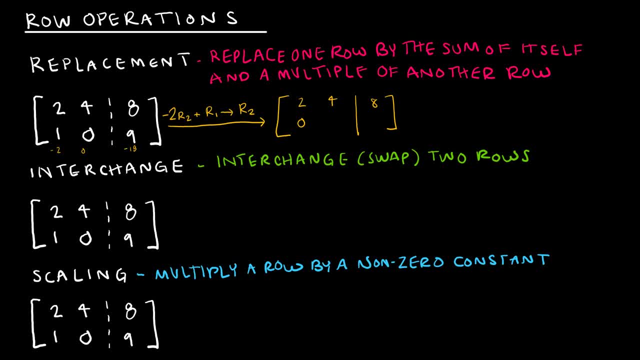 to row 1, that's going to give me 0 here, and then 0 plus 4 gives me 4 here, and negative 18 plus 8 gives me negative 10 here. so that would be an example of replacement. interchange just means to swap two rows. so again, I'm going to show. 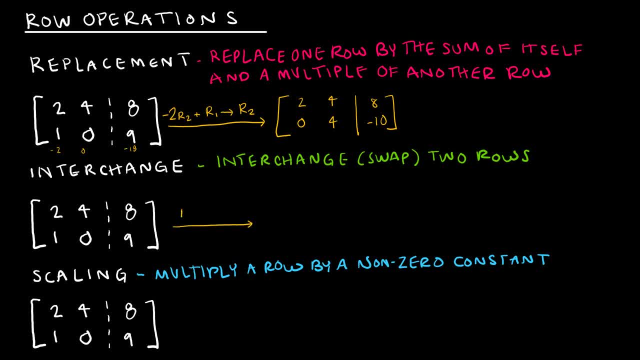 you the proper notation. if I want to replace row 1 and row 2, I'm going to use an equal sign, essentially with an arrow on each side. so this is telling me I'm swapping row 1 for row 2. so if I do that, then this would be 1 0, 9, and this would 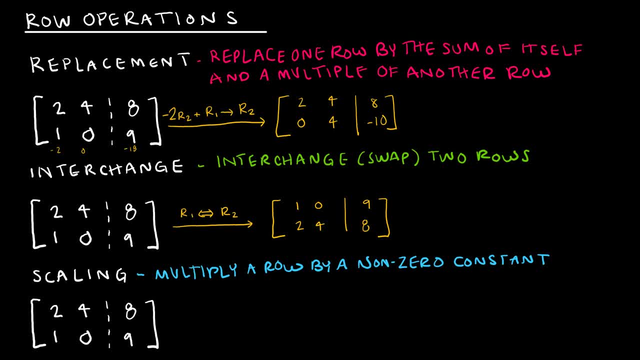 be 2, 4, 8 and lastly we have scaling. scaling again is just multiplying a row by a nonzero constant. so a great example here would be row 1. obviously these are all multiples of 2, so I can just say: let's take half of row 1, and again I have to. 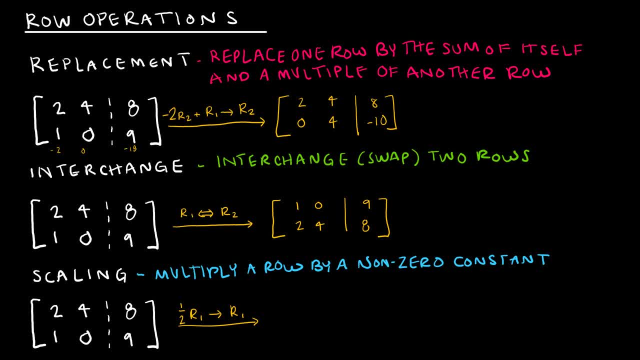 put my new target row, which is again row 1. so that means, and again I can't use division, division is not one of the row operations. so I can't say R 1 divided by 2. I have to say half of row 1. so half of 2 is 1, half of 4 is 2, half of 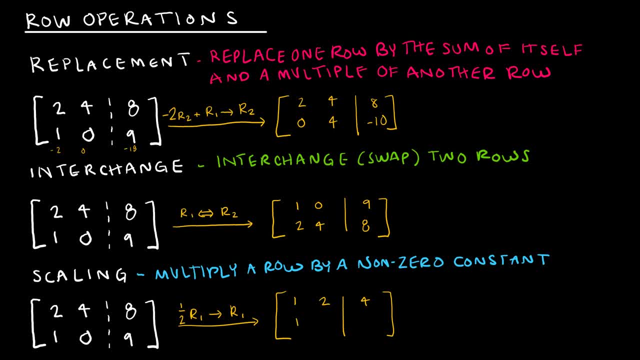 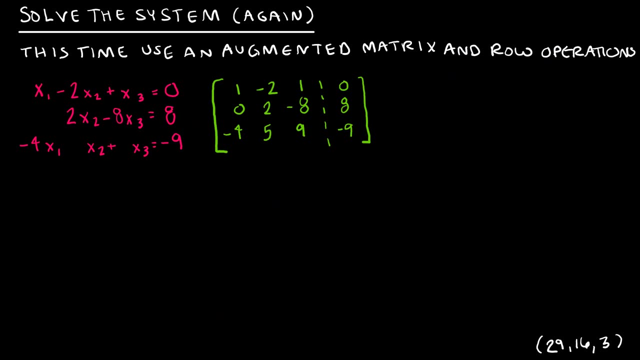 8 is 4 and again nothing has happened to row 2. that stayed exactly the same. so those are the three row operations and the proper way that I would like you to show your row operations. this question should look familiar to you, because we just solved this in the last video using elimination. now, obviously, I want. 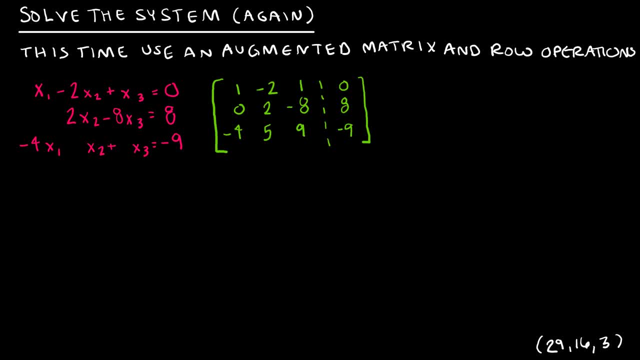 to use augmented matrices and row operations. now we haven't really talked enough about a good strategy, so really I just want you to sort of follow along with me and I'm not going to give too much of the strategy away, because I'm going to talk about that in the next video and the video after that. so all of 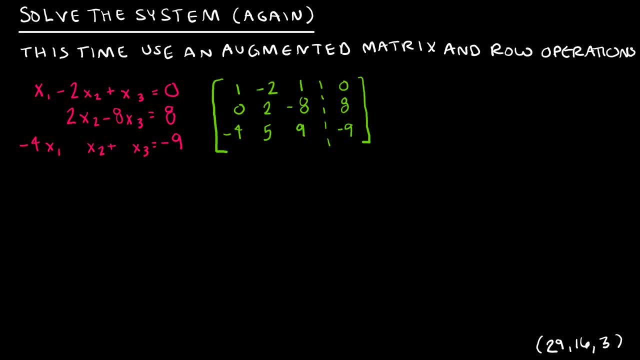 section 1.2 is about. here's how to go about solving a system in the best, most efficient way possible. and then what happens when you have variables that don't have a value. but for now you're just going to kind of follow along with me and do the best you can, so thinking. 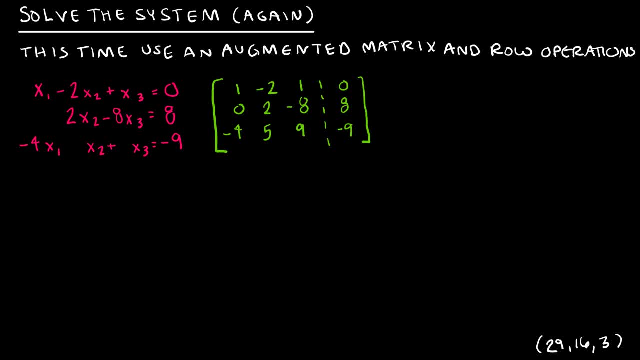 about this in terms of elimination, and, again, we haven't talked about this yet, but what I would like is I would really like these values to all be ones, and then anything that's not there, I like to have them be zeros. so we definitely need these three values to be zeros, and, whether or not you use these, 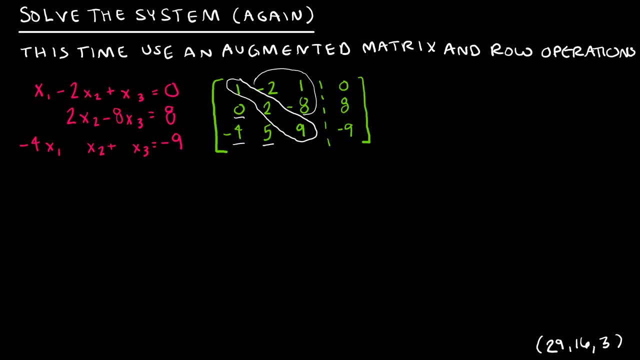 three values to be zeros is up for debate, and I'll let you decide the best way that you want to go about that. but for now, you're just going to do it the way I want to do it, because I'm the one making the video. so what I'm going to do, 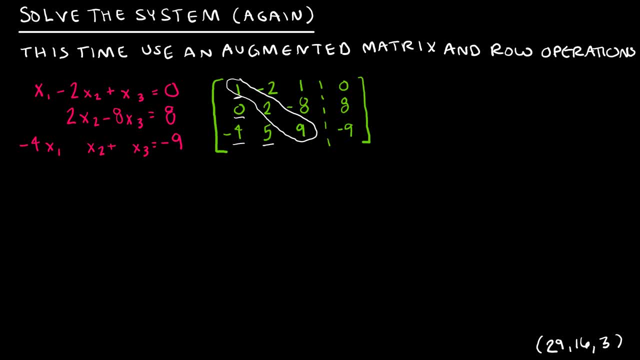 first is because I already have a 1 here where I want it, and I already have a zero here. I'm going to focus first on: let's choose a different color. this guy right here. I want that to be a zero. so every time I have a value of one, I want everything below that to be a zero, and 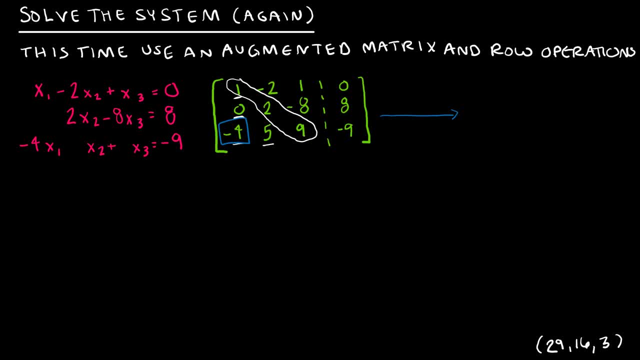 we'll talk more about that later. so how am I going to make negative four into one, I'm sorry, into zero? I would have to add positive four, so negative four plus positive four, zero. how can I add four to that? well, I have to use one of my three row operations, the easiest row operation. 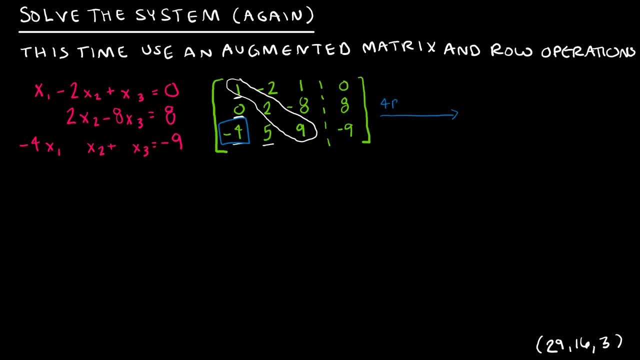 is to then take positive four times row one, because four times one would give me positive four. adding that to negative four gives me zero. so I'm going to add that to row three to be my new row three, and that gives me- and notice, this is row. 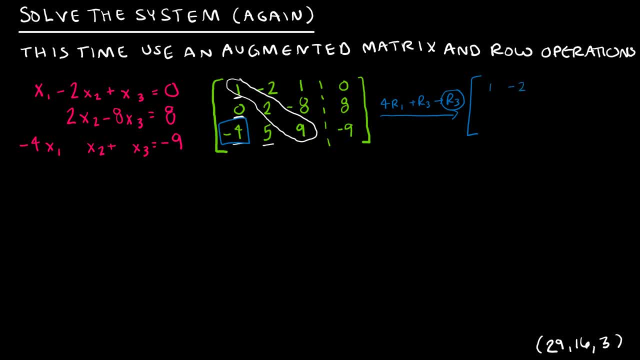 three is the target row, which means this guy doesn't change, this guy doesn't change. row three is the only one that changed. so what changes? we take four times row one, so four times one plus negative four, four times negative two plus five and four times one plus nine and four. 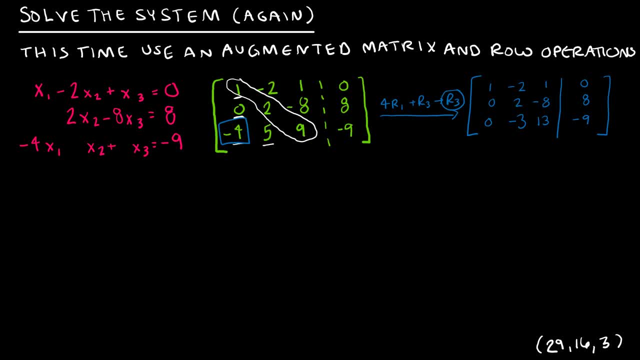 times zero plus negative nine. so that's all for my first step. now what I want is I'm going to focus on this guy. what do I want that to turn into? I want it to turn into a one. well, when I'm just taking something down to a one, not a zero, but 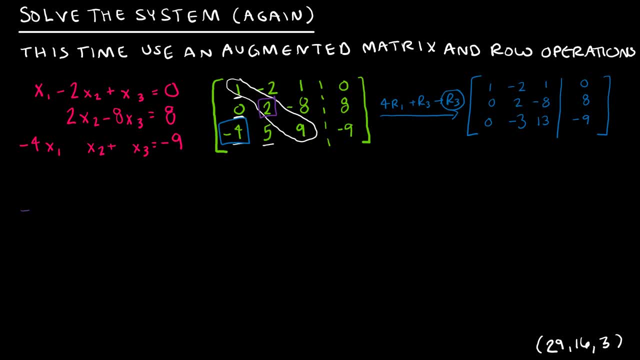 if I'm taking something down to one, usually I'm going to use scaling, and that's what I'm going to do here- is, I'm just going to take half of my row two to be my new row two. so I'm just taking half of row two. so that means 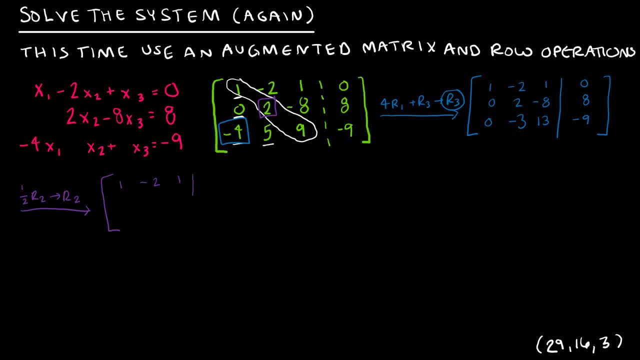 row one is the same, row three is the same row two. I'm just taking half. so half of zero is zero, half of two is one. half of negative eight is negative four. half of positive eight is positive four. now what I need- let's see if I've got another color- is this guy to be a zero. so again, when I'm 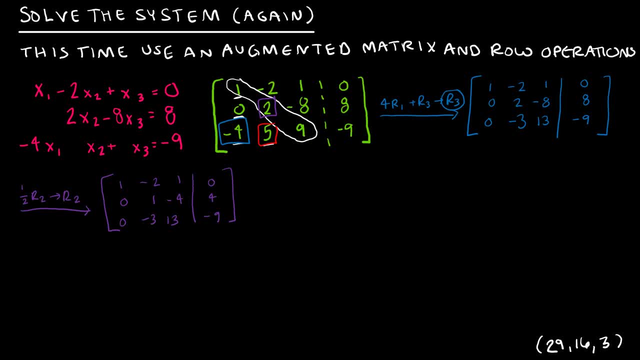 turning something into a zero. usually that means I'm going to have to use interchange, where I'm multiplying and adding together. now I could obviously use row one, but if I use row one, this guy is going to become problematic because I'm going to probably end up screwing up my zero, and I don't want to. 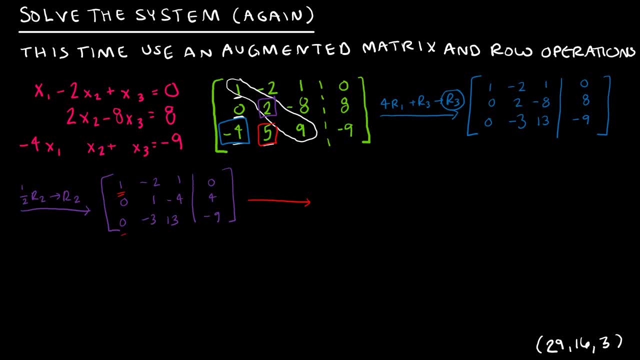 backtrack and have to redo work. so what I want to do is I want to use row two to help me to get row three how I want it. so I'm going to take three times row two and add it to row three to get my new row three. so what is that? 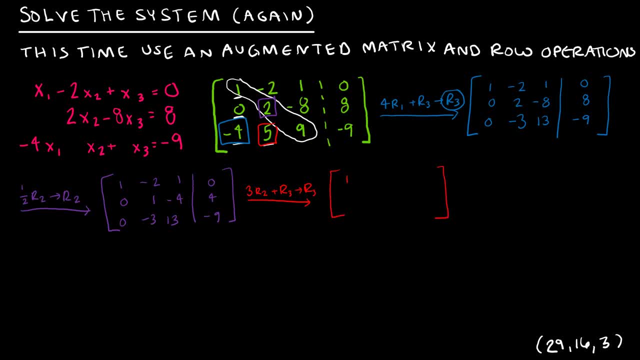 going to do. that's only going to change row three. so row one: one negative two, one zero. row two: zero, one, negative four, four and row three. I'm taking three times row two, so three times zero plus zero, three times one plus negative three. three times negative. four is negative. twelve plus thirteen is. 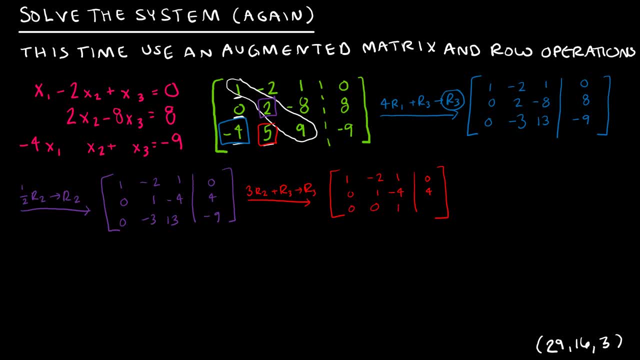 one and three times twelve, I'm sorry, three times four is twelve, plus negative, nine is three. so far, so good, because remember that's what this means is that x3- you know zero, x1 plus zero, x2 plus one- x3 is equal to three, and that's what I want. all right, let's. 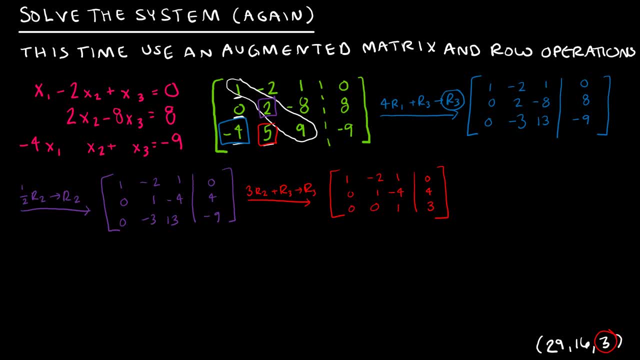 continue on now. what I want is: this is where you kind of make a choice, and again, we'll talk more about this in the next video, but I really have to let you in on the secret here. this is essentially called a triangular form, and we'll talk. the book will call it triangular form, and it's triangular. 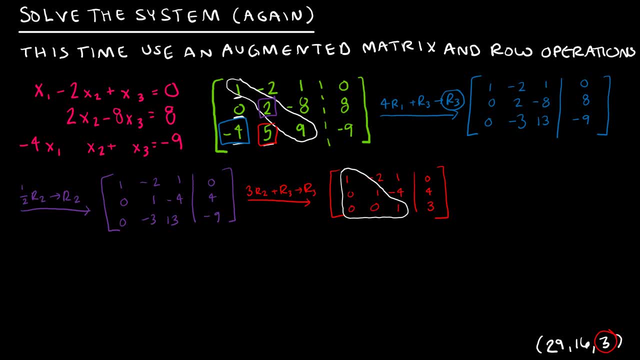 because we've got the triangle and we've got the square, and we've got the ones and we've got the zeros, and quite often we don't have all ones here. we just have the zeros where the zeros are supposed to be, and then the ones we can. 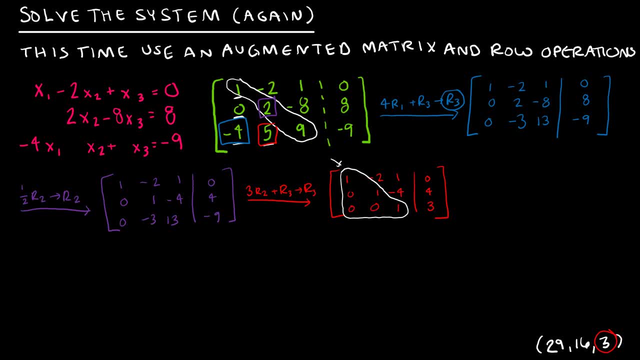 deal with later. that's what your book calls triangular form. this is actually Gaussian elimination. and then going on to the next step, which is making all of these zeros, is Gauss Jordan. but again, it doesn't matter what you call it, because it's still the same thing. so from here, I have a choice to make. I can either 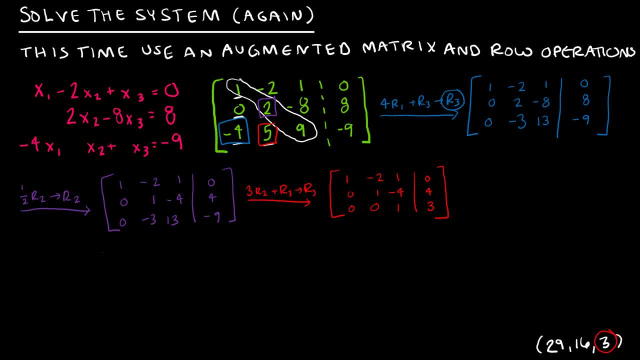 and your book probably shows it to you. this way, I can either take that this equation and turn it back into an equation: x 1 minus 2x 2 plus 1 equals 0, and then 1x 2 minus 4x 3- whoops, I forgot my- x 3 equals four, and then 1x 3 equals 3. so from here, obviously, I can either use that equation like this and take that equation and take that equation and turn it back into it, and then go through this, and then you'll end up with 2放 이걸 monzo Henry's top We Versus x-1 minus 2x, two plus one, x2 plus 1 equals zero, and then 1x 2 minus 4x3- whoops, I forgot my. x3 equals 4, and then 1x 3 equals 3. so from here, obviously, I give it some sort of meaning, and maybe I have an incarnation as well, and then we're done. I talk about the. 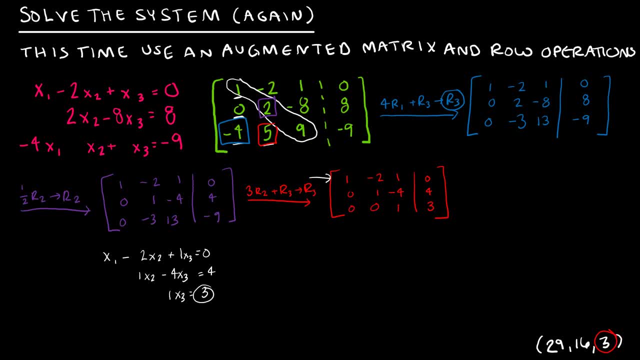 can use back substitution and I can say: well, I've already found that x3 is equal to 3.. I can very easily say: x2 minus 4 times 3 equals 4, which gives me x2 minus 12 is 4, which gives me x2 is. 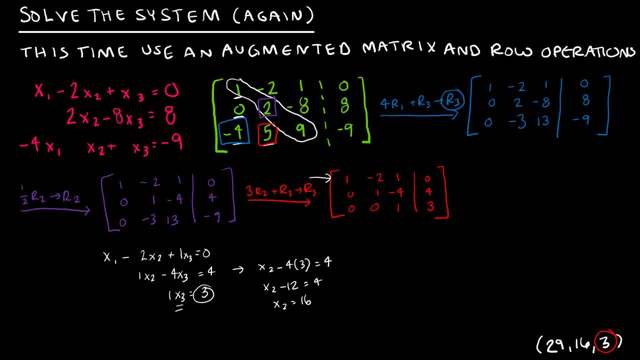 16.. And again, that's the correct answer. And then I can take 3 and 16 and substitute those back into my original equation. So x1 minus 2 times 16 plus 3 equals 0.. x1 minus 32 plus 3 is 0. x1. 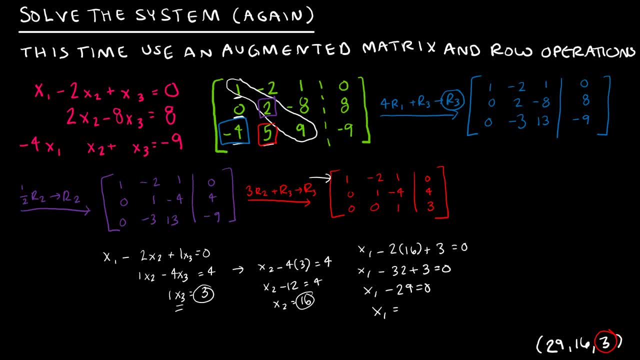 minus 29 is 0.. x1 is 29.. And again, I've solved the equation. So this is using back substitution And instead you can also- and for now, since we're not focusing completely on the correct algorithm, you could also do whatever- 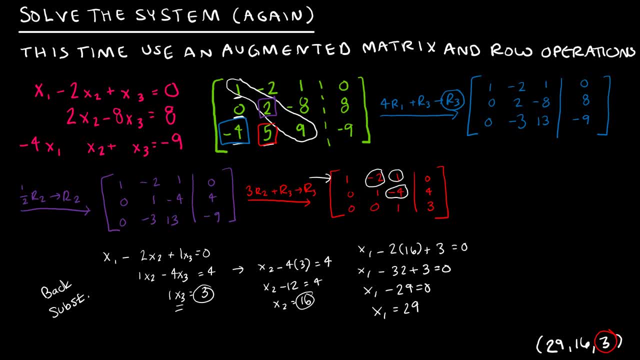 row operations were necessary to turn these values into 0. And that's the way that I prefer to do it. But again, for the sake of this video not being 37 minutes, let's not. If I do it that way, what happens here is I would end up with my three solutions, And that's why I like it. 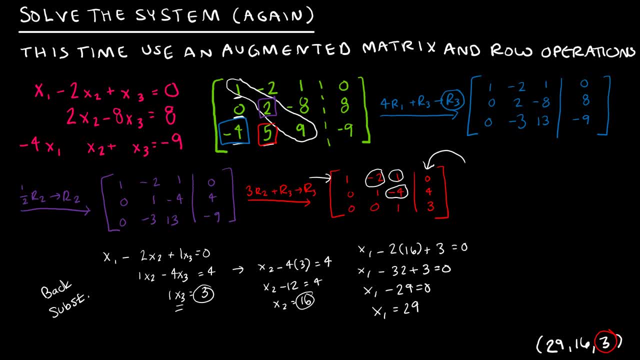 is, I might as well just keep going. So I'm going to keep doing row operations until I've actually solved the system. But for now we can see that we have solved the system again using an augmented matrix and row operations and in this case also back substitution. 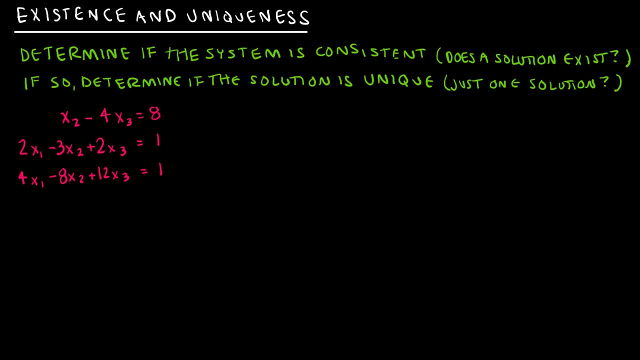 You're going to see the question of existence and uniqueness pop up quite often throughout the course, And when we're talking about existence, we're essentially asking: is the system consistent or does a solution exist? And uniqueness means if a solution exists, then it's consistent, And uniqueness means if a solution exists, then it's consistent, And uniqueness means if a solution exists, then it's consistent. 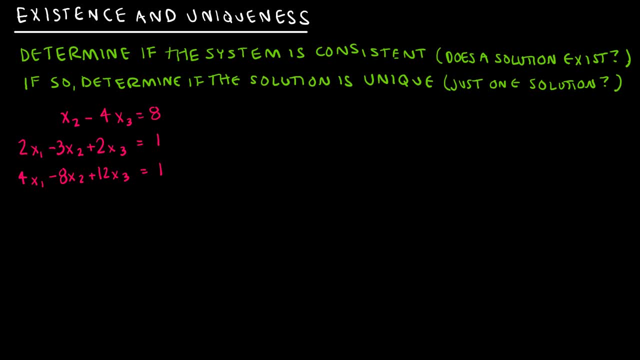 So, whether a solution does exist, is it unique meaning? is there one solution or are there many solutions? So let's take a look at this one together And, again, we're trying to determine. so far, up to this point, we have only looked at consistent systems with one solution. 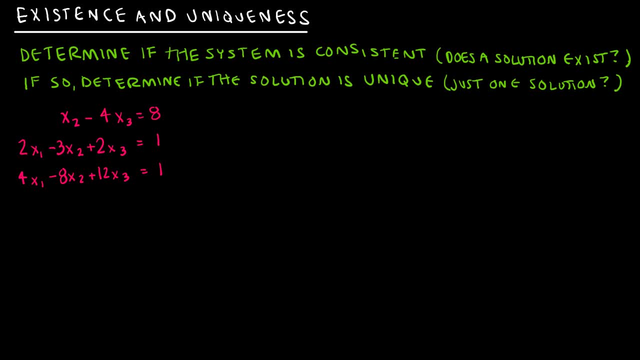 So let's take a look at maybe one that isn't like that. First thing I'm going to do, as always, is write my matrix: 0, 1, negative 4, 8.. 2, negative 3.. 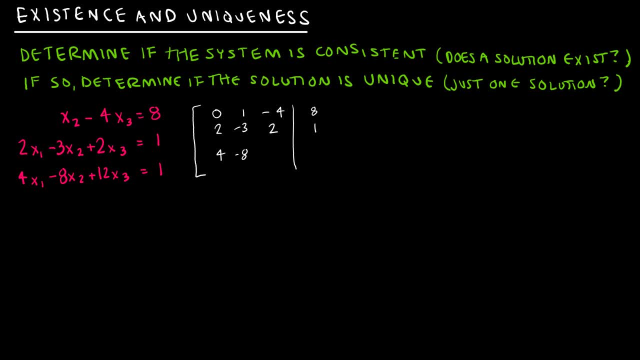 two, one, four negative eight, 12, one And, just as we talked about before, I really want this column to end up being ones, but I've got this glaring issue right here with this zero, So I can't have a zero there. 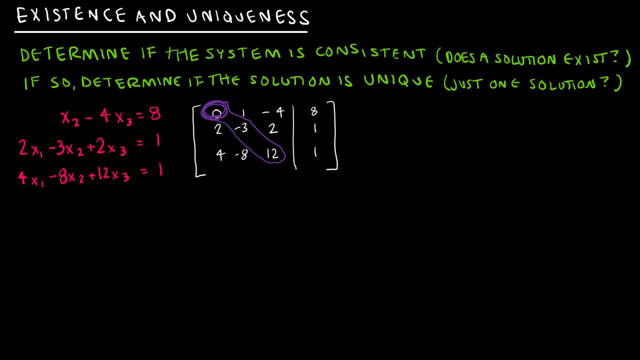 I have to have, and in the next section we'll talk about all the terminology. but essentially right now I'm just telling you we have to have something there other than a zero. So the easiest thing I can do is essentially swap R2 and R3 with one. I'm sorry, nope, just kidding. 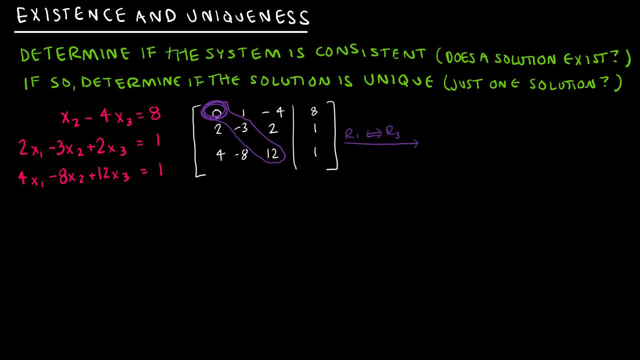 Swap R1 and R2, or R3, but I'm gonna go R1 and R2.. So if I swap R1 and R2, I really haven't done anything except swap them, interchange them, and now I have zero, one negative four, eight. 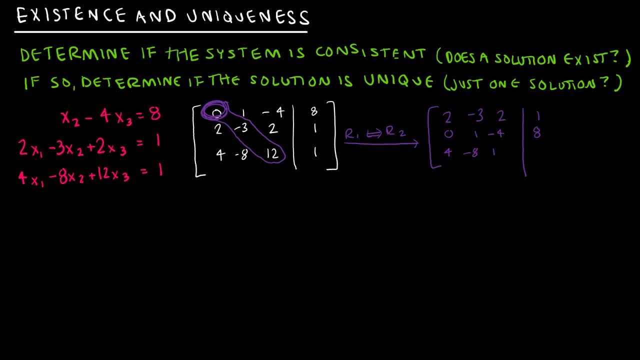 and then my second row and everything else stayed exactly the same. So again, the purpose of that is that I didn't like that. I didn't have some value here. Now what I'm going to do is I'm going to try to get that to be a one. 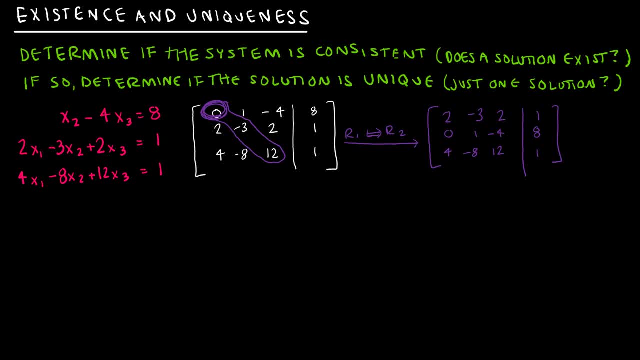 So, according to the correct algorithm, I don't need it to be a one, I just need it to not to be a zero. I like to have a one there, So that's what I'm going to do next. So I'm just going to take half of everything in row one. 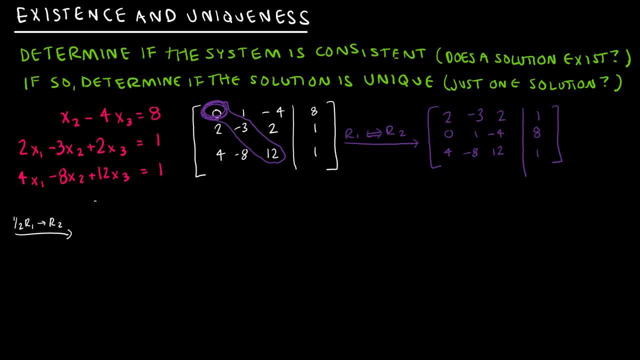 to be my new row one. So that's using scaling, And so I'm going to get one negative, three halves, one. oops, one half, and this stays the same, And, oops, that's a positive four. 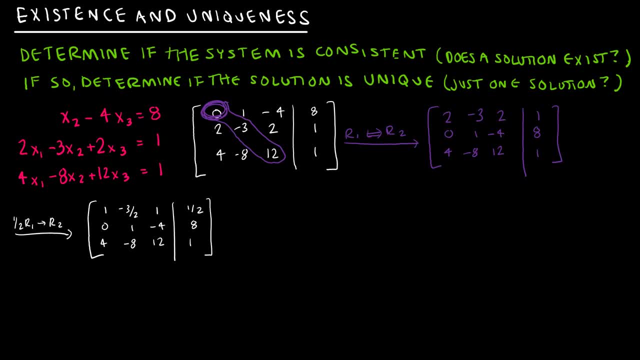 Four negative eight: 12, one Okay. So I have a one where I want it, but what I don't have now is I want this to be a zero, because once I have a one, I want everything below it to be a zero. 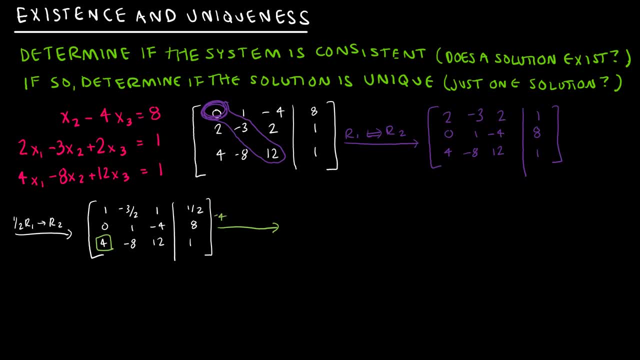 So I'm going to take four times- sorry, negative, four times row one, because I need a negative four to cancel out my positive four plus row three to be my new row three. So row one remains the same. Row two remains the same. 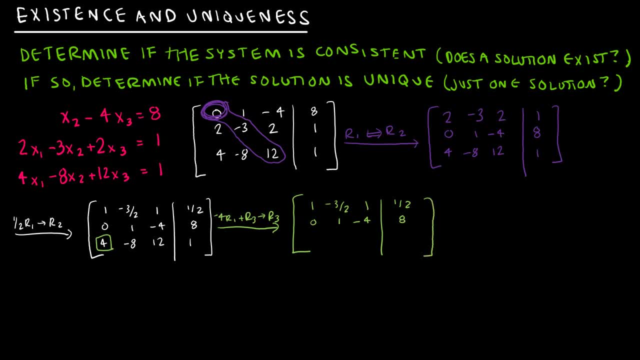 And row three is now negative four times row one plus row three. So that's going to give me a zero here. It's going to give me 12 halves. So six and negative eight is negative. two Negative four times one is negative. four plus 12 is eight. 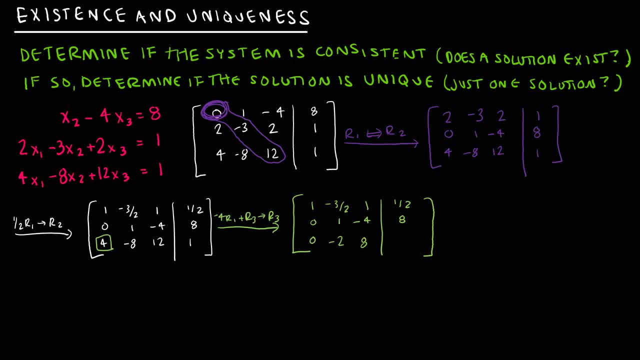 And then negative four times one half is negative two plus one is negative one, And then negative four times one half is negative two. Now, I would focus on making this a one, but it already is, So I'm going to focus on making this a zero. 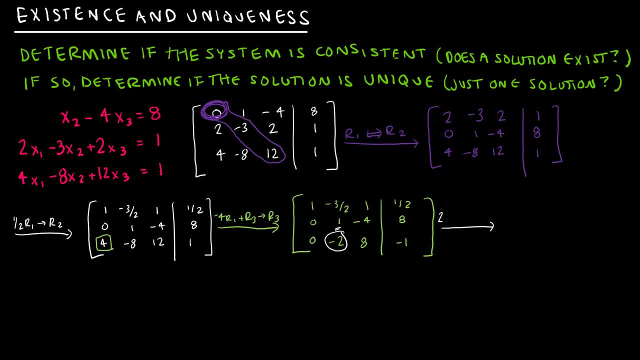 So to make that a zero, I'm going to take two times row two plus row three to be my new row three, which means row one is the same, Row two is the same And row three is the same And row four is the same. And row five is the same, And row six is the same, And row seven is the same, And row eight is the same, And row nine is the same, And row 10, Amul- is going to be the same. We're going to simplify. 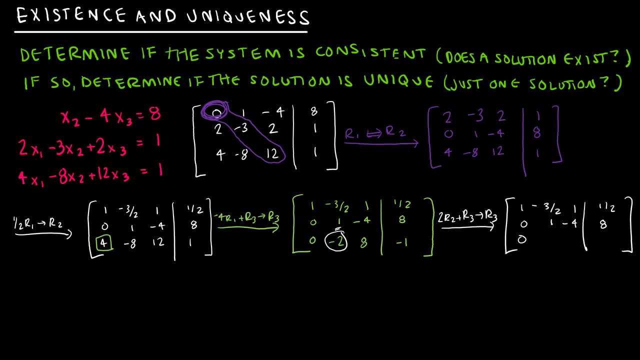 Okay, now there are two times row two. Oops, all my fat fingers down here making little marks. two times row two plus row three, So that gives me a zero here, That gives me a zero here And that gives me a 15 here. 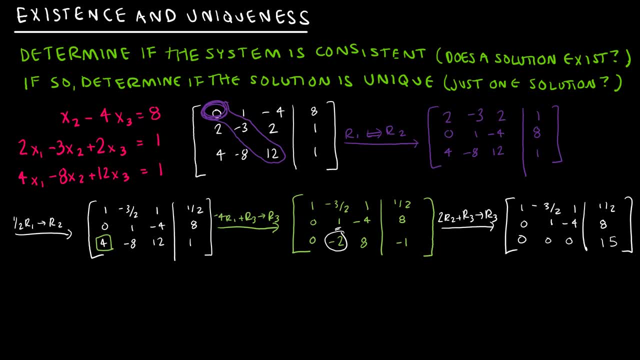 So we're going to stop right now, because remember what this means. This says zero X, one N, zero. Athos plus 0x2 plus 0x3 is equal to 15.. Well, that is impossible. and because it's impossible, 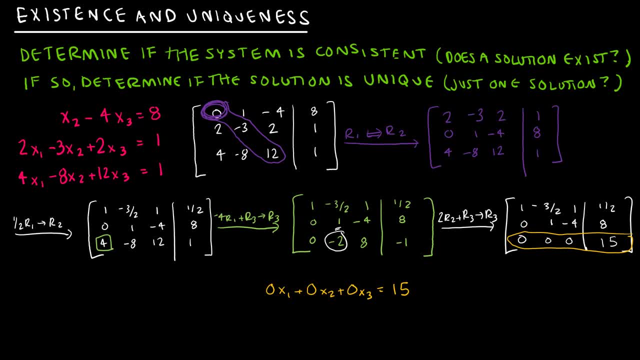 that means no, there is no existence. so this is an inconsistent system. So no solution. and is it unique? Well, obviously we don't have to check that if there is no solution. so inconsistent system in this case. So here's a question for you to try on your own and again, 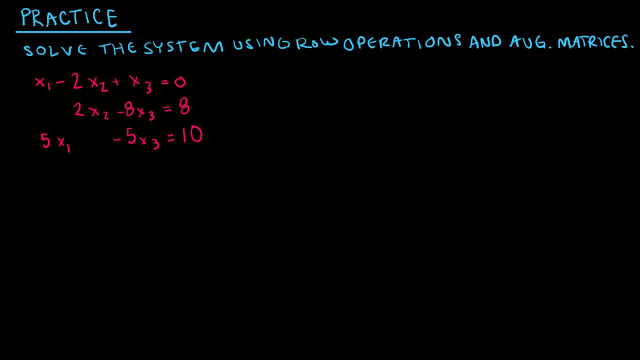 be very patient with yourself. just do the best that you can. we're just learning how to do this in no time at all. this will just come a second nature to you. but since we're just getting started again, just be kind to yourself. do the best that you can try this question on your own when 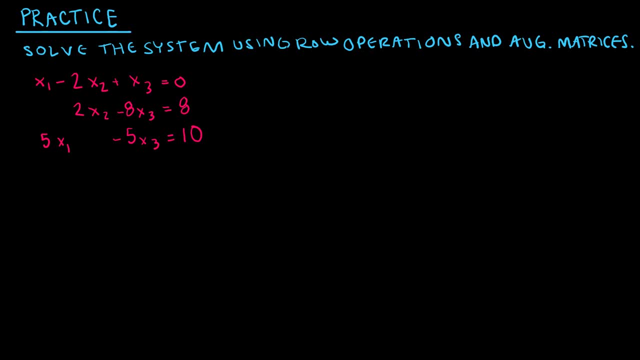 you're done. press play to see how you did So again. the first thing I would do is write this as an augmented matrix. So I have one negative two, one zero, I have zero, two negative eight, eight, and I have five zero negative five, ten, and I already have a one exactly where I want it. and 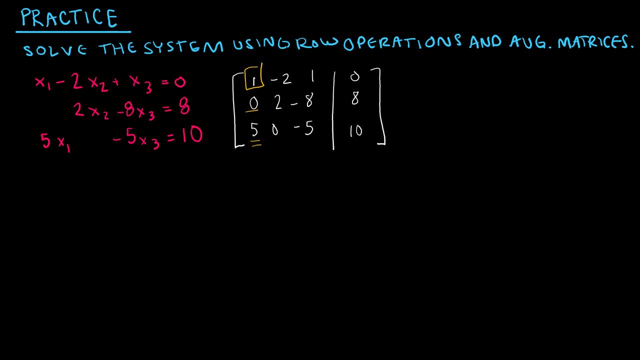 I have a zero just below it, and I would like that five to be a zero as well. so that's the first thing I'm going to do. How do I get rid of five? I have to add negative five, so I'm going to take 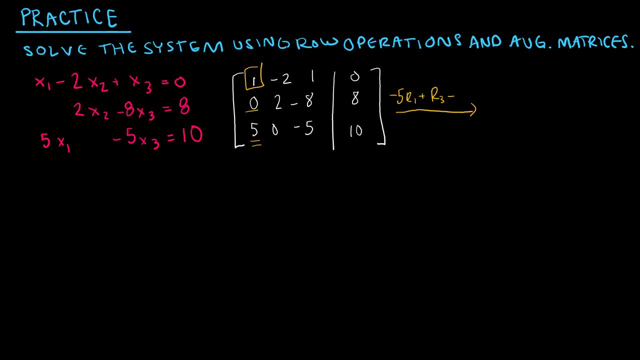 negative five times: row one plus row three, to be my new row three. Notice that means row one remains the same, row two remains the same, but actually- and I'm going to cheat a little bit- I'm going to do something to row two at the same time, just because I noticed that these are all even. 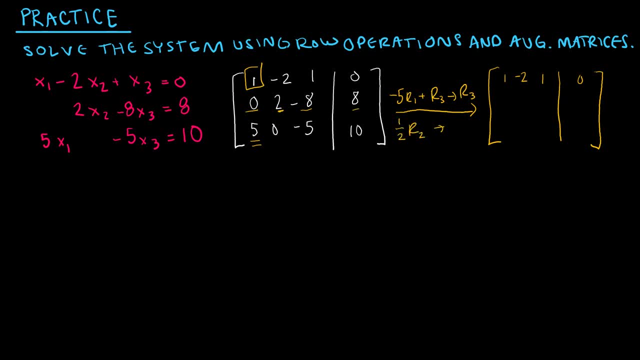 so it's okay for me to take half of row two to be my new row two in the same step. so this is going to be zero, one, negative three, negative 4, 4.. And then the negative 5, row 1 plus row 3.. So negative 5 times 1 plus 5.. Negative 5: 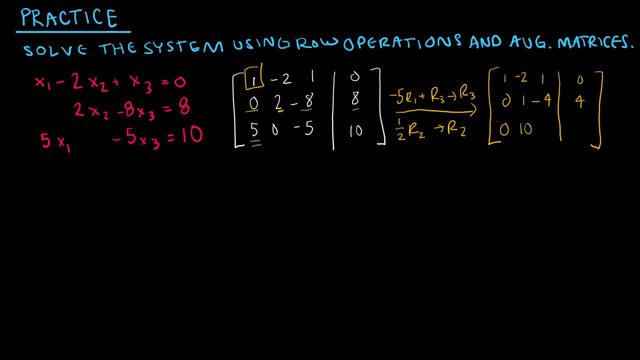 times negative: 2 is 10 plus 0.. And then negative 5 times positive: 1 is negative. 5 plus negative 5 is negative 10.. And then negative 5 times 0 is 0 plus 10 is 10.. So that was a good first step, or? 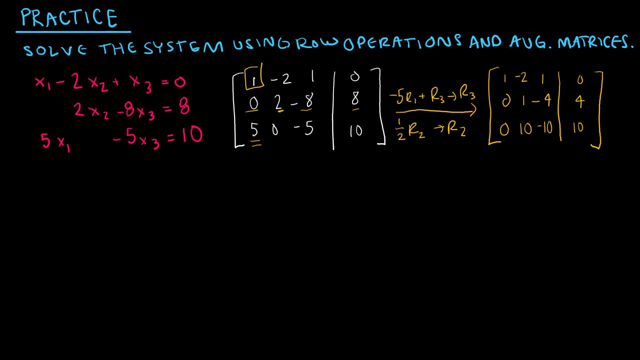 first two steps, I guess, since I cheated just a little bit- And again I have one where I want it and I've got zeros below it, And I've got one where I want it here, But notice, I want a zero above and below that as well. So again I can do two separate steps. Typically, I would start with. 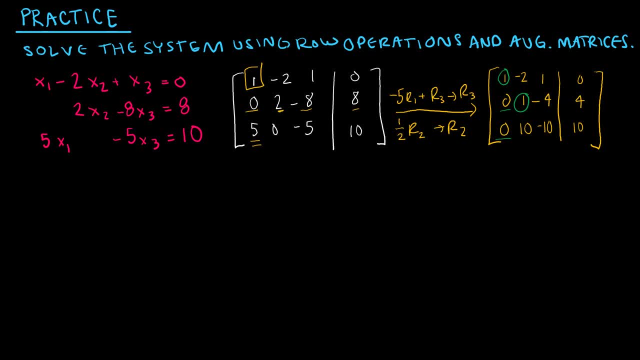 that one on the bottom, Or I might even say: look, everything is divisible by 10.. And so I might divide everything by 10. It's really up to you. Again, we don't have an algorithm yet, So I'm. 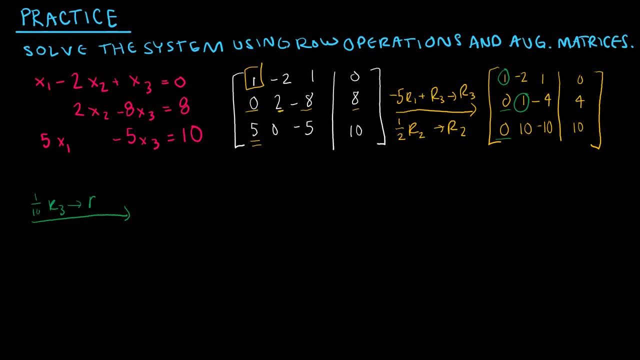 just going to take a tenth of row 3 to be my new row 3 and see where that gets us. And that gives me 1, negative, 2, 1, 0.. 0, 1, negative, 4, 4.. And 0, 1, negative, 1, 1.. So now I again have the ones. 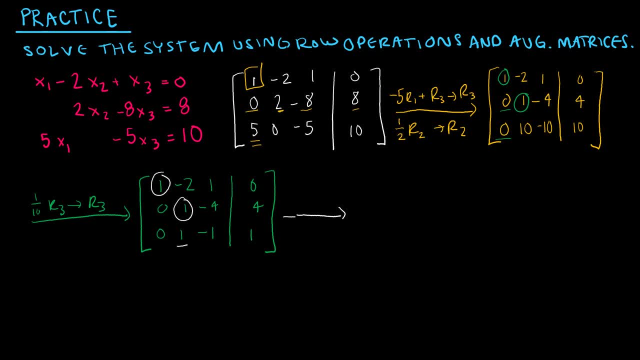 where I want it. I need this guy to be a zero. So let's do row 2 minus row 3.. And I'm going to take a tenth of row 3 to be my new row 3.. Row 1 is the same, Row 2 is the same, Row 3 is 0 minus 0,. 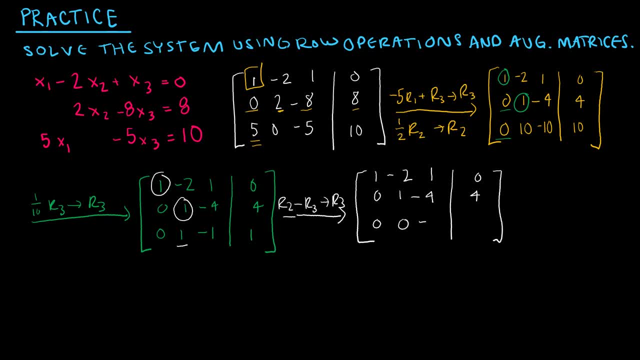 1 minus 1, negative 4 minus negative 1, 4 minus 1.. And then I'm going to- because obviously these are both divisible by 3, let's change that. And then I'm going to take a tenth of row 3 to be my. 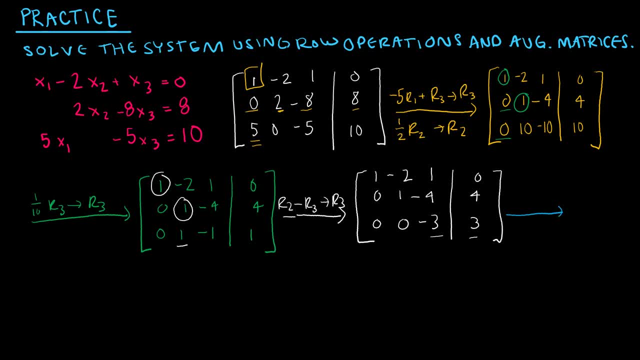 new row 3.. And I'm going to shift these into given colors again And I'm going to take a third of row 3 to be my new row 3.. And again right now, because we don't know the correct algorithm. 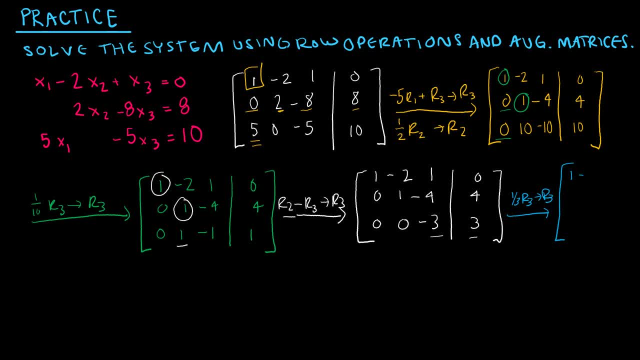 if you do it in more steps, if you do it in fewer steps, everything's fine. right now We're just learning, So again, don't be hard on yourself. Then 0, 1, negative 4,, 4.. And then 0,. 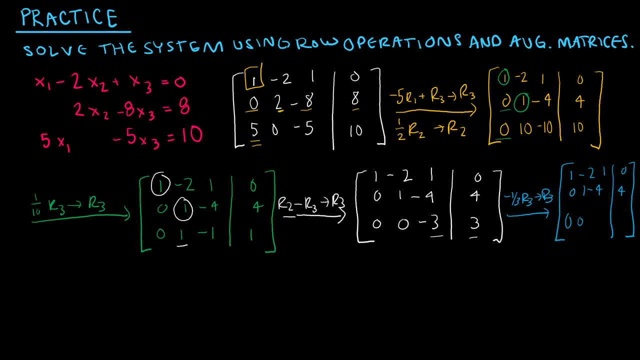 zero. I'm going to take- sorry, negative, one-third. so that's positive one, negative one. Now I'm going to continue. I would like the negative two to be a zero as well. So I'm going to take two times row two and add it to row one, to be my new row one. 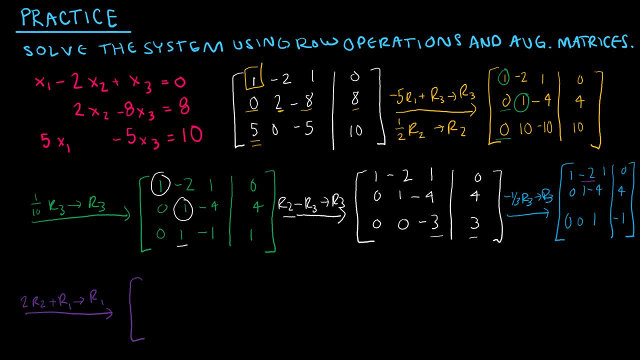 So that gives me two times zero plus one, two times one plus negative, two, two times negative, four plus one and then zero. Oh no, just kidding. eight Two times four is eight plus zero is eight. And then my second row. I haven't done anything to. 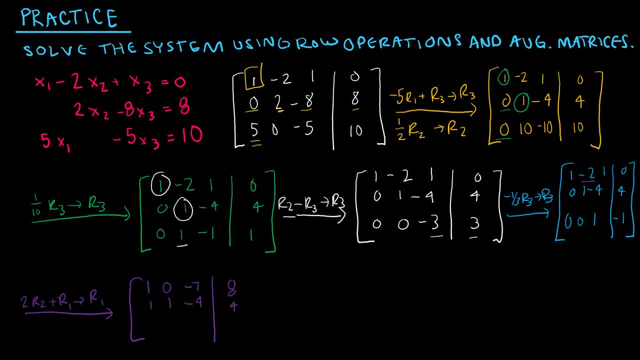 And my third row: zero, zero, one negative one. So I'm getting there. Oops, I magically just put a one there for no reason at all. So this guy's what I want. these guys are this guy's what I want. these guys are this guy's what I want. 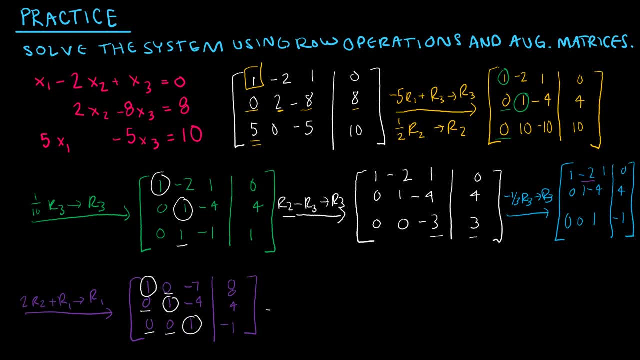 and I still have to work on the negative seven and the negative four. So let's do that. I'm going to do both of those on the same step here. So to get row two to have a zero, I'm going to take four times row three plus row two to be my new row two. 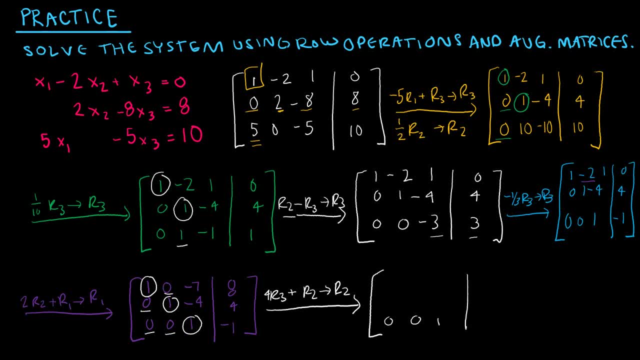 So let's keep this guy exactly the same. Row two is zero. zero plus one is one. Four plus negative four is zero, negative four plus four is zero. And then, to get my new row one, I've got a negative seven. 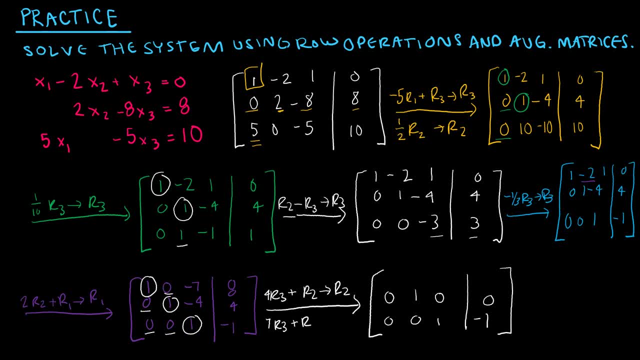 So I'm going to take seven times row three plus row one to be my new row one. So now that gives me one zero, zero, and then I've got negative seven plus eight, which is one. So my solution as an ordered pair is: one zero, negative one. 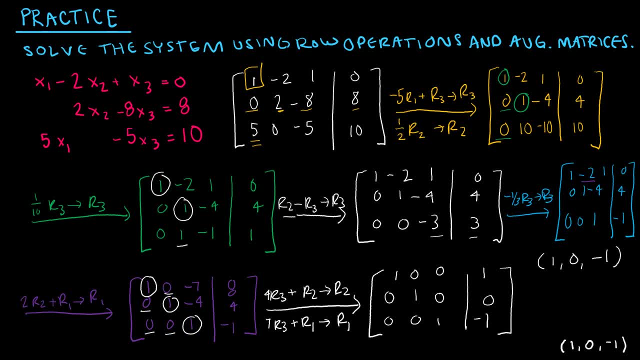 And again, that is the correct solution. So if you got that, great job. If not, that's okay, We're going to keep working at it. 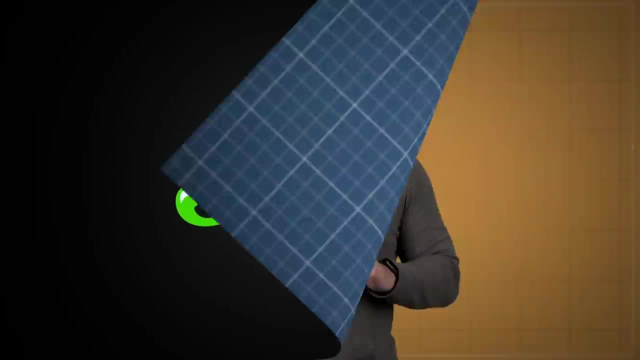 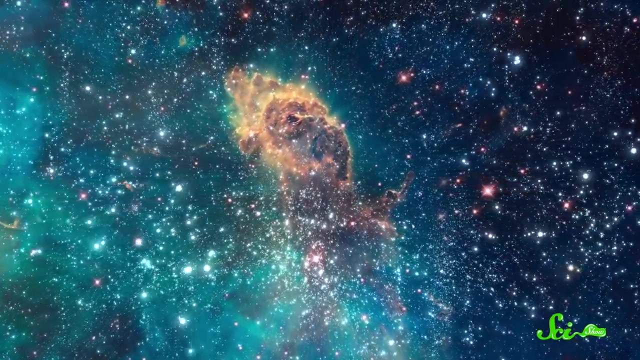 The universe is vast, complex and awesome. Despite hundreds, if not thousands, of years of scientific endeavor, there's still so much we don't know about it. And that point was hit home last week with results out of Fermilab, a particle physics. 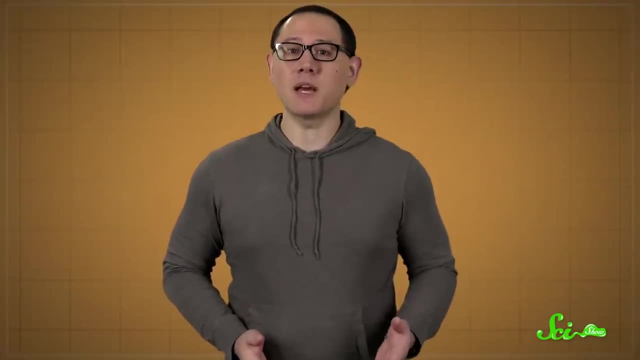 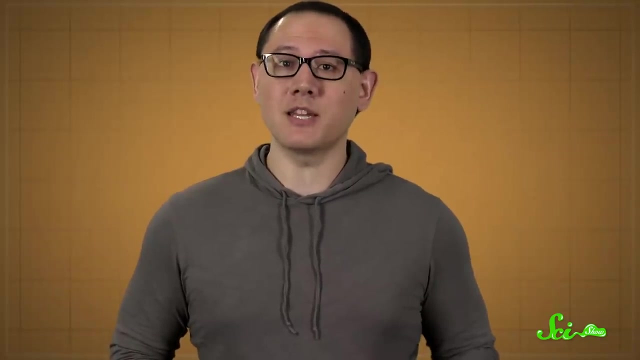 lab in the US state of Illinois. In their experiments, tiny subatomic particles called muons disobeyed the laws of physics as we know them, And, if the results hold, the only logical explanation is that there are kinds of matter and energy out there that physicists either don't fully understand or don't yet. 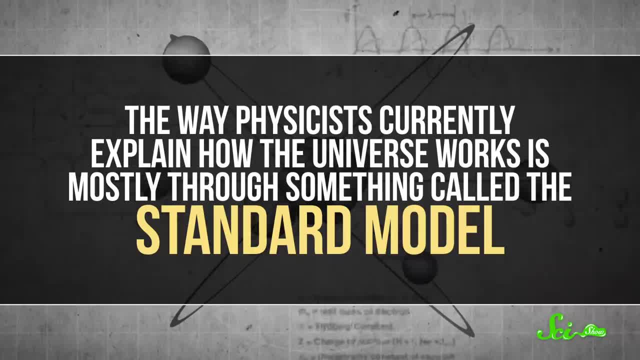 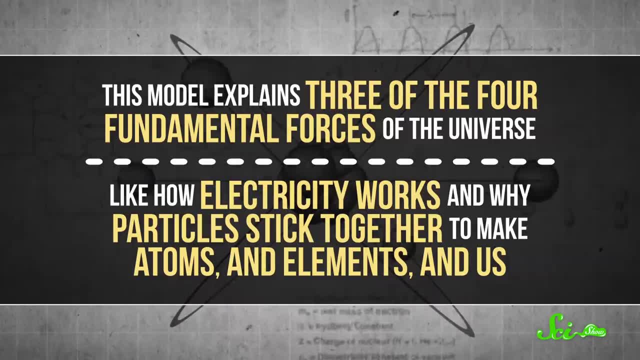 know about The way physicists currently explain how the universe works is mostly through something called the Standard Model. This model explains three of the four fundamental forces of the universe, like how electricity works and why particles stick together to make atoms and elements and us. 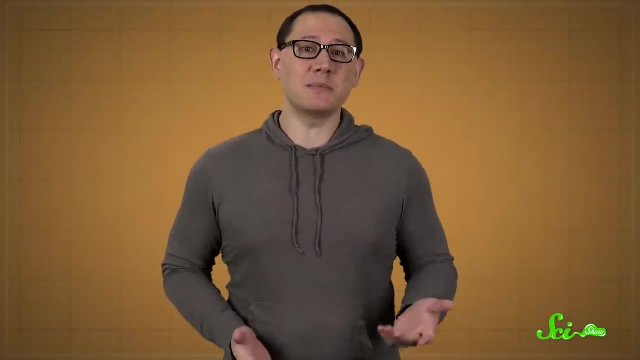 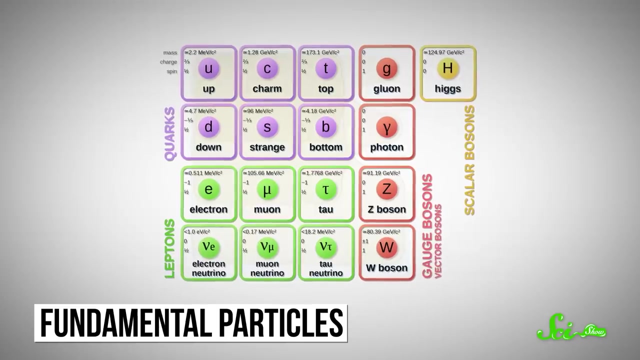 The only one it doesn't cover is gravity, because, well, gravity doesn't seem to matter to subatomic particles. Besides, we have the whole theory of general relativity, for that The Standard Model also describes 17. building blocks, called fundamental particles, that make up everything.